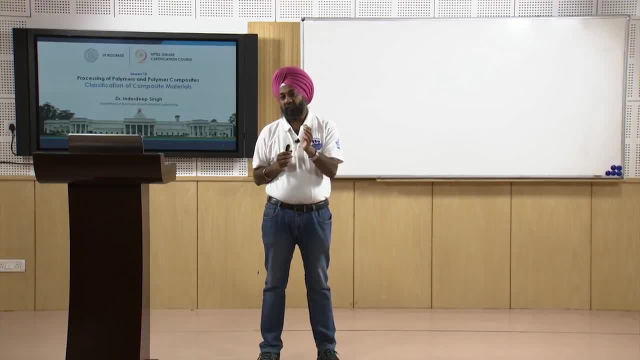 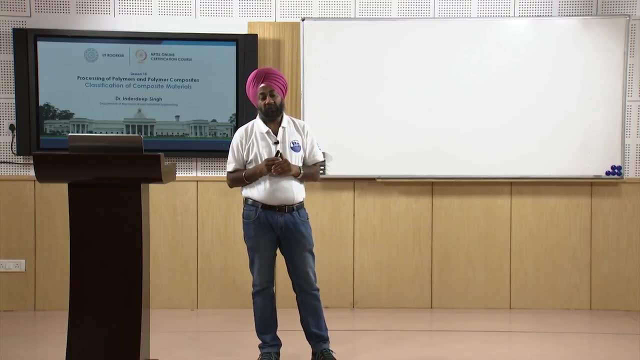 information, very basic information. and then we have covered the different processes that are used for processing of polymers. if you remember, we have covered the casting process as applied to the plastics processing. then we have covered thermo forming, we have covered extrusion, we have covered compression molding, injection molding also. 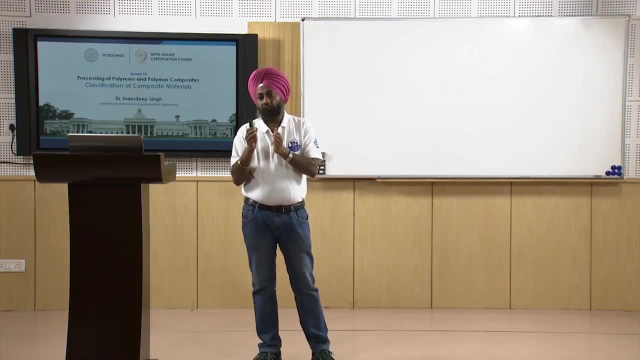 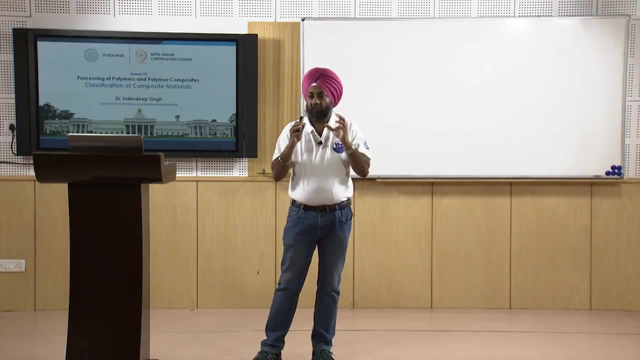 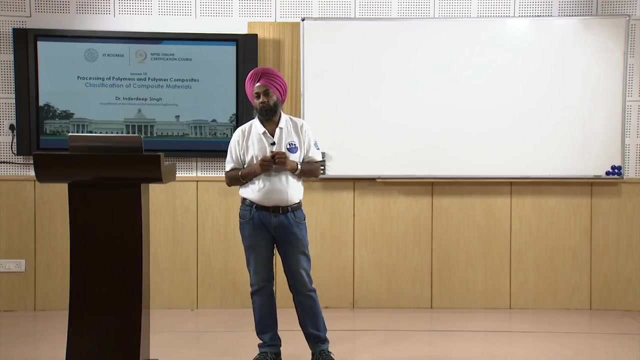 we have covered ah other processes like blow molding, which are very commercially used, and transfer molding we have covered. so by now i think all the learners have a fair amount of idea that what are the processing routes, techniques, fabrication processes that are followed for processing of polymers. 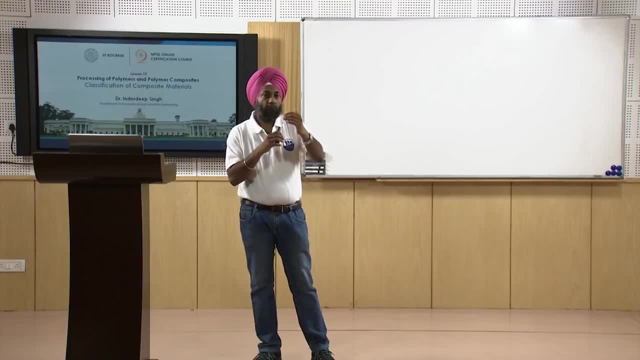 Now, in the last session we have shifted our attention from neat polymers to polymer based composites and in the last session i have just given an introductory aspect of the composites. that is, what is a composite material actually? we have seen two definitions of composite materials and we have tried to understand that there are broadly two constituents in 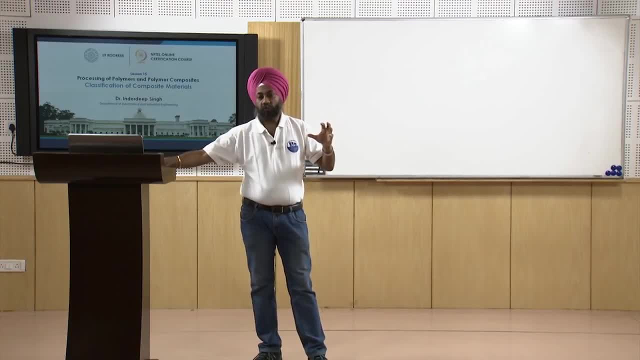 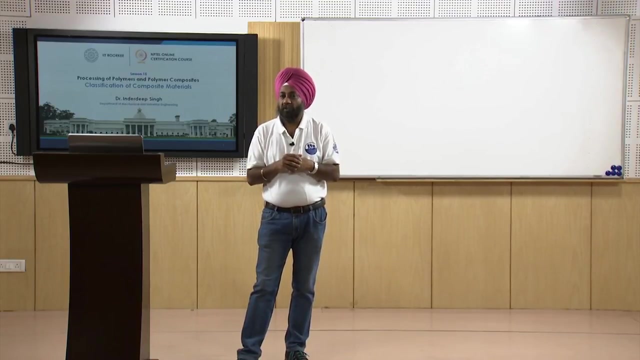 a composite material. now, what are these two constituents? that these two constituents are one ah matrix, another one is a reinforcement. so these two constituents are combined together to make a third material which has properties, which is the best combination of the best properties of both the constituents. so we have tried to understand the basic concept. 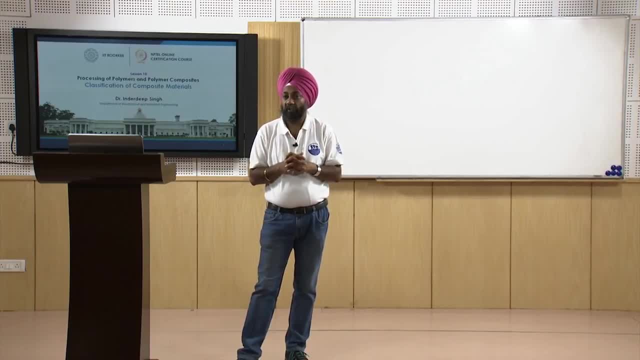 of composite material that why do we need to develop a composite material? what is the need for developing a composite material? and we have also understood what are the advantages of the composite material. and we have seen that for light weight application, composites have been developed word by word. 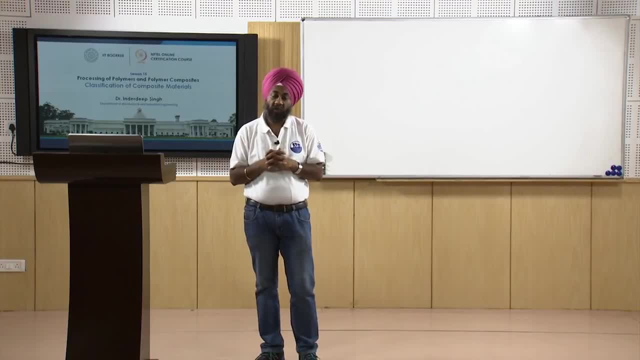 And they find lot of applications in the aircraft industry, automotive industry and there are number of other applications like biomedical industry, sports equipment, even household items are today being made by composite materials. so last class focused on the basic aspect of composite, that why do we need to combine the two different materials which are physically 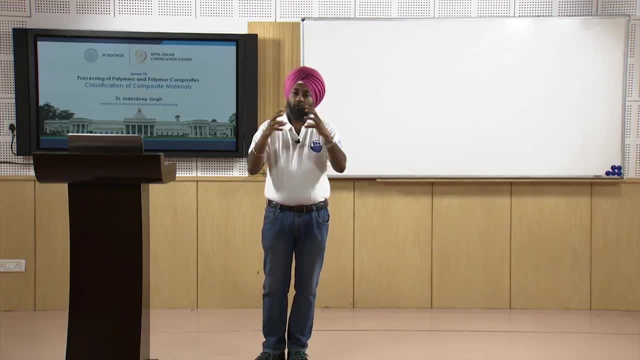 different, which are, which are chemically different, to form a third material. so that was the basic concept. Now we have taken an example of the RCC structure, or our roofs also, in which we have metallic rods and concrete. that what is the purpose of combining the metallic rods and the concrete? 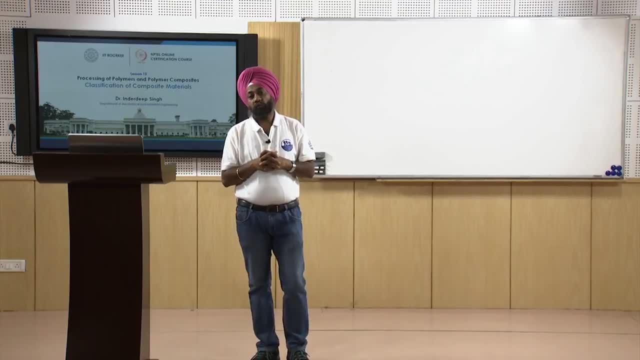 to make a structure. today, our focus would primarily be on the classification, because composite material is a very big family. there are a lot of research- ah, research scientists or engineers are working in the field of composite material, but we have to see that what is the broad classification? 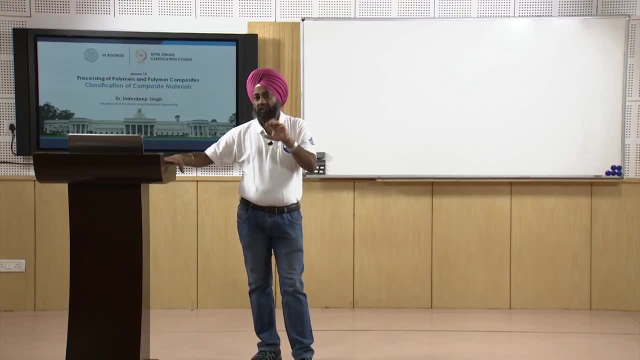 How the composites can be classified now, classified means that what is the bigger family, that is, the composite, then dividing them into its individual sub families and then the further sub families, so sub sub family. so we have to see how the composite materials are classified. for all composite materials, for all practical purposes, two constituents will remain same. 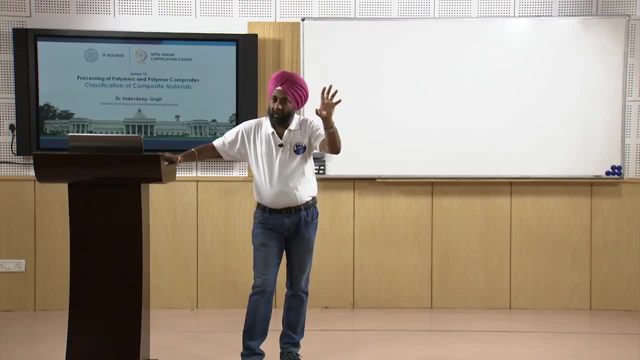 that we have discussed in the previous class. that is, one will be the matrix, another one will be the reinforcement And the matrix will have its own role to play. in the last session we have seen what is the major role of a matrix. it provides the bulk to the composite. it is a continuous phase. 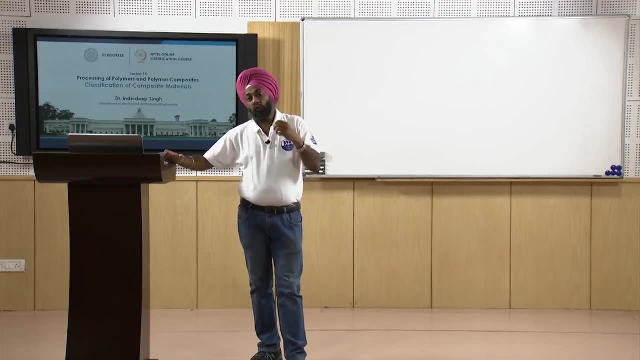 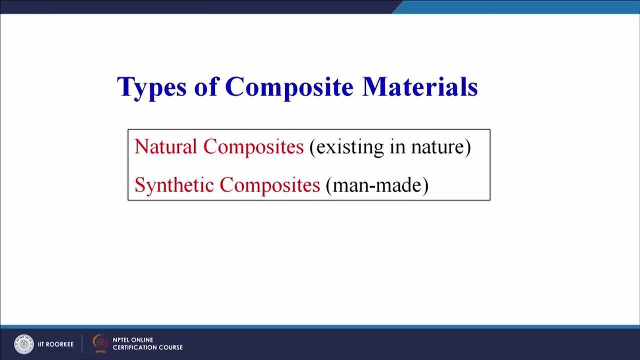 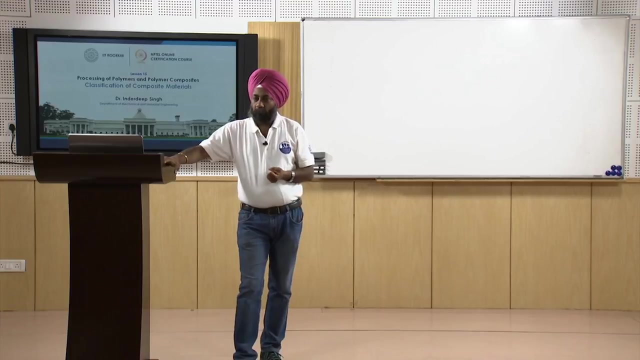 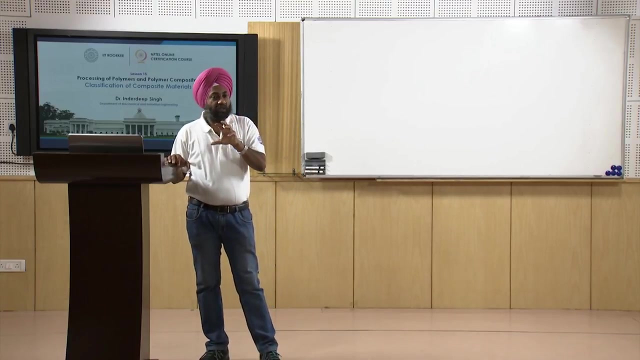 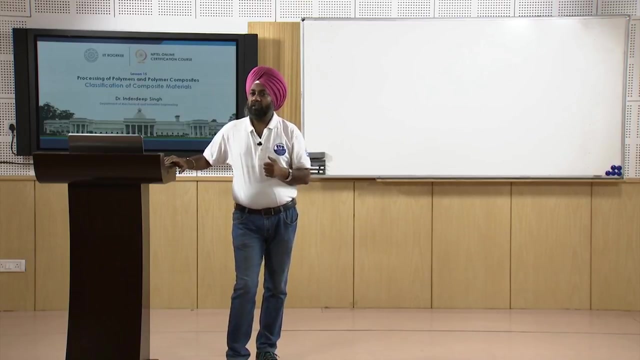 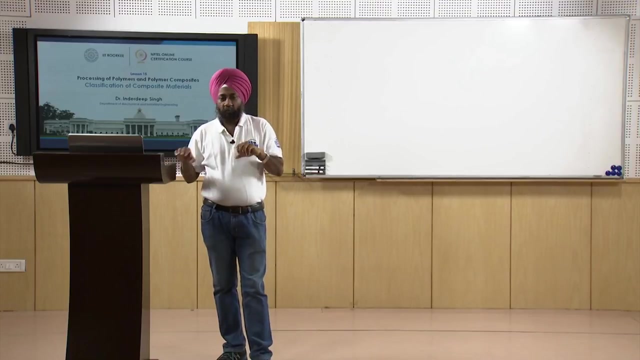 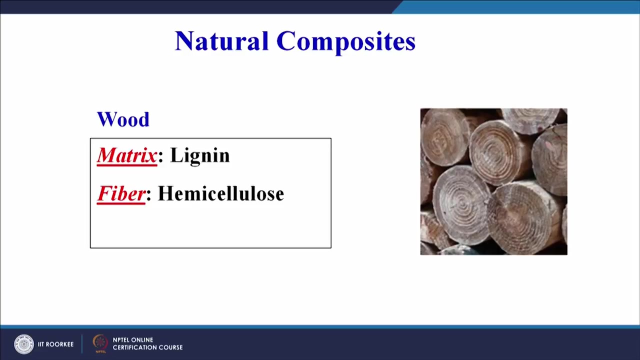 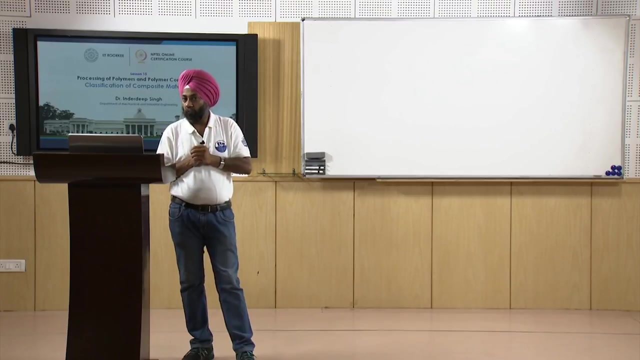 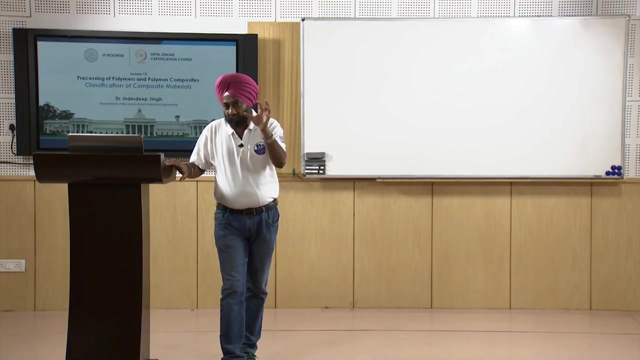 as well as it supports the fibres or the reinforcement. moreover, it leads to the transfer or it acts as a medium for the transfer of load when the load is applied on the composite material among the fibres that are used as the reinforcing elements. Why the properties are different? because of the constituents. 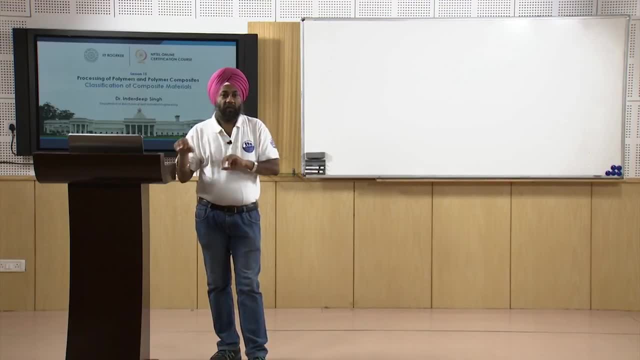 And these constituents may be present in relative amount, somewhere one constituent may be in larger amount, the other may be in a slightly smaller amount. so basically, we need to understand that there are two or three major constituents that add up to make wood and that defines the properties of the wood. and in the last class, or last session, if you remember, we have 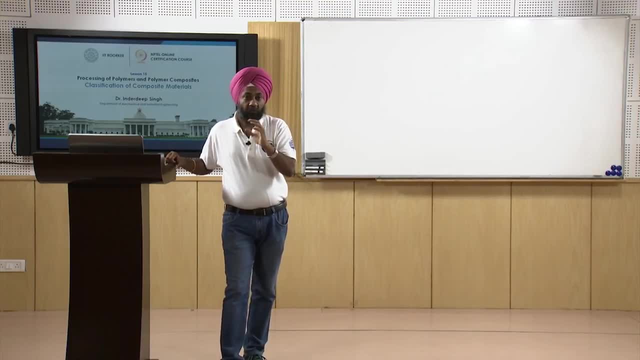 clearly try to understand that, how we can differentiate between an alloy and a composite. Estimate m, MEB, So composite, and what are the three major criteria which a material should satisfy to be classified as a composite material. so that is a very common question, if you will tell somebody. 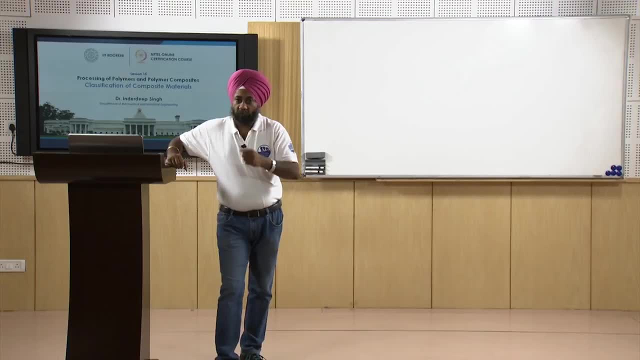 i have undergone a course on polymer composites or i have information on polymer composite, the first question that you will be asked is how to differentiate between an alloy and a composite, and how to differentiate between a polymer and a polymer blend, how to differentiate between a polymer blend and a polymer composite. so these are some issues which are usually 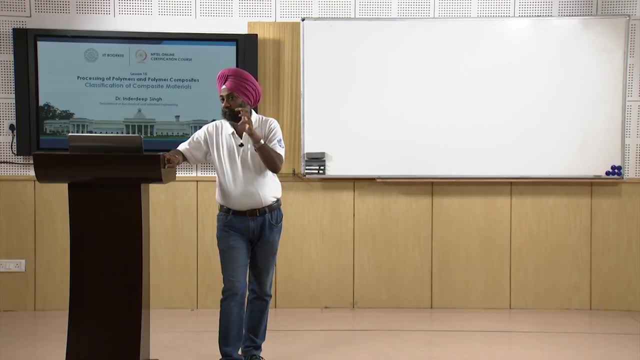 asked from the students, and that answer you should frame in your minds after going through this session, particularly the previous session, in which we have tried to see that how you can classify a material as a composite. classify means what is the criteria based on which you will say that this is a composite material? and if you remember the five percent, ah ah. 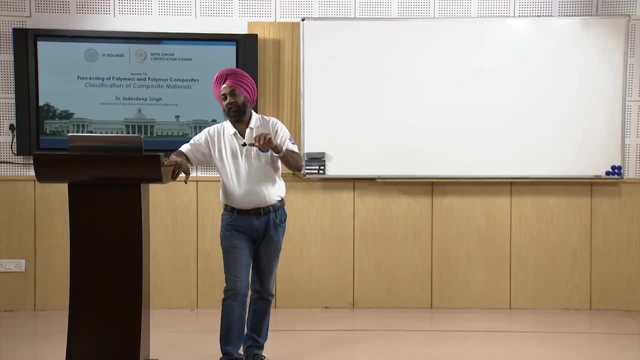 critical limit was there that both the constituents should be present in appreciable amounts, but the lower constituent or the lower quantity constituent must be above at least five percent. so that was one condition. other condition was that the two constituents do not chemically- ah are soluble into each other. they are insoluble. 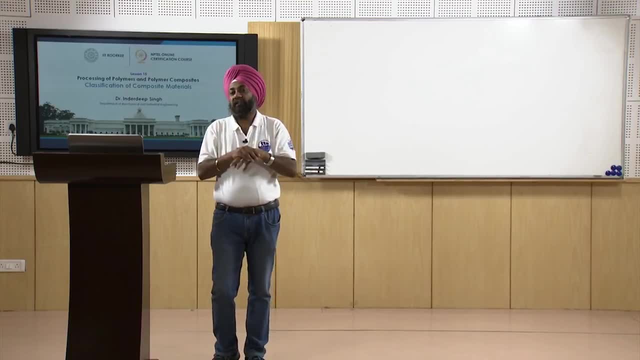 into each other and there is a interface that separates the matrix and the reinforcement. so there are certain guidelines, certain hints which will help you to differentiate an, an alloy, an alloy, from a composite material. so that is the information that you should always keep. and here also somebody may say: bring a different. 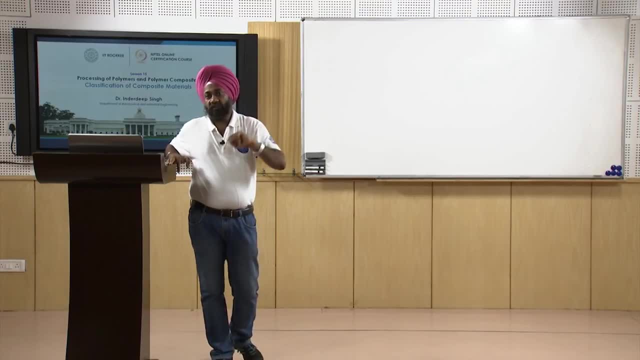 material which has two or three constituents and may ask you Whether we can make this or we can classify this material as a composite material. you should look at those criteria. if those criteria, ah for those criteria- are being satisfied, then only you can say that, yes, we can classify it as, as a, or we can term it or name. 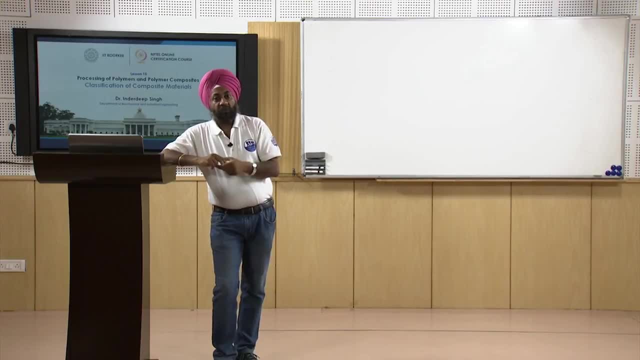 it or define it as a composite material. now there can be ah question that you have a subscription to the compound Enforcer Woods recipe for processing. if you do not have cost charge, liquid et cetera, dept what should be your business knowledge if you want the benefit for your students. 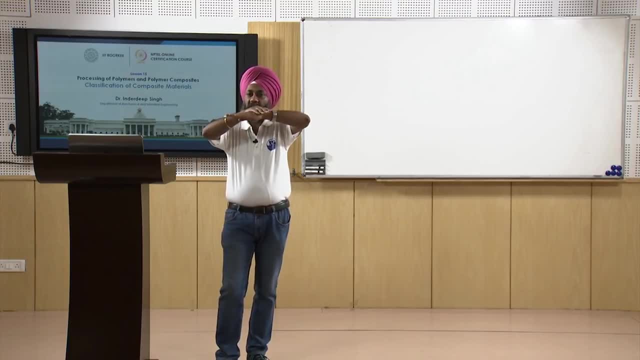 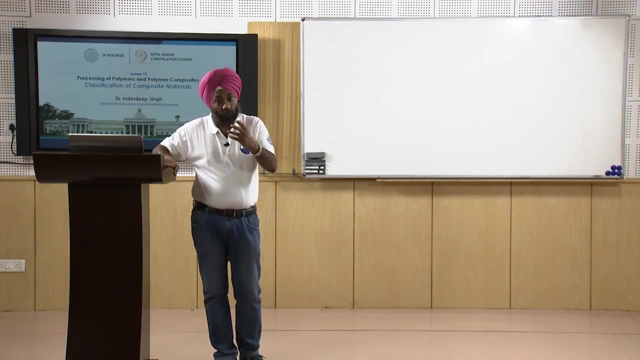 substrate or a base material and you do a coating on that base material. now somebody may say: now there are two constituents, one is a coating, another one is a substrate. this can be called as a composite material. no, we cannot say that it is a composite material. why? because in one has to be a continuous phase. so here there are two different constituents. 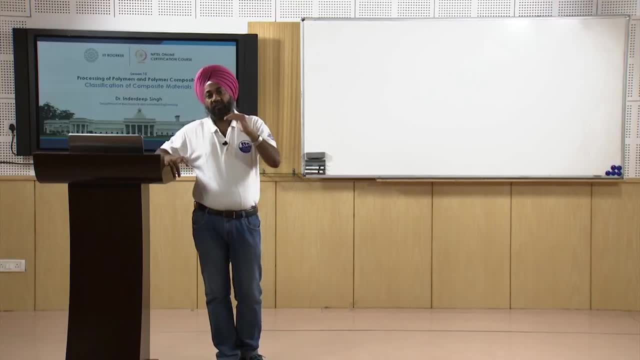 but there is no continuity of any phase in this thing. so we can say, yes, it is a coating on a substrate, but we cannot classify it as a composite material. but there is no continuity of any material, of any of the constituents, so there are few, we can say grey areas where 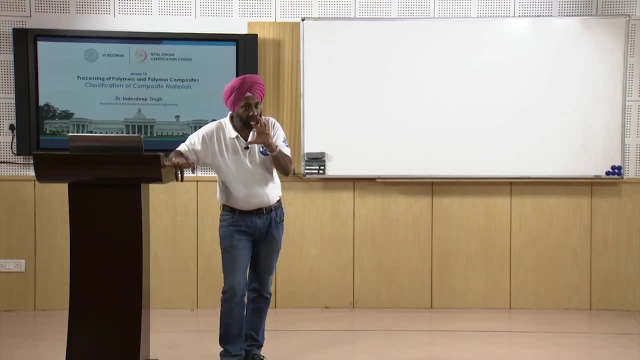 we need to focus and try to understand that. what exactly are the composite materials? and there is lot of, we can say, debate going around to classify or define composite materials clearly so that ah learner has clear idea that this is a composite material and this is not a composite material. 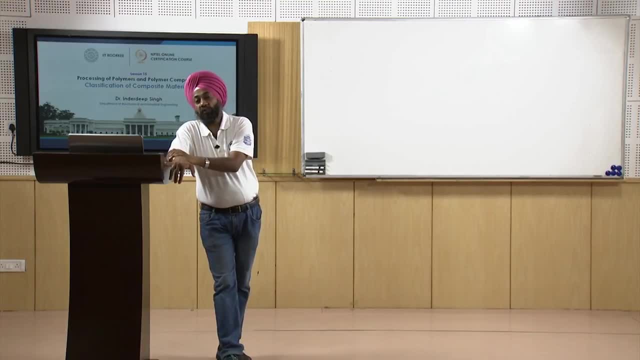 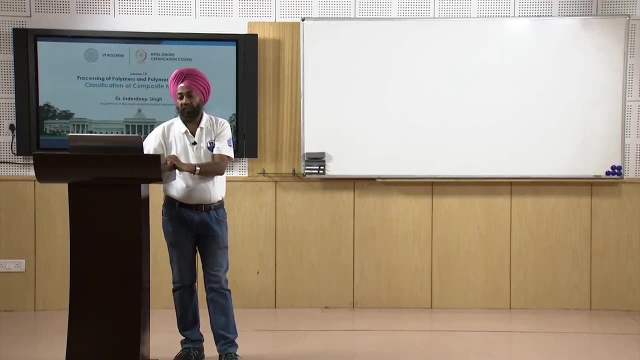 so that is the purpose of defining, or ah, going through this todays session in which we will see how to classify a material. so first classification on your screen: one is natural composite, another one is synthetic composite. so if you are asked that, what are the different types of natural composites? 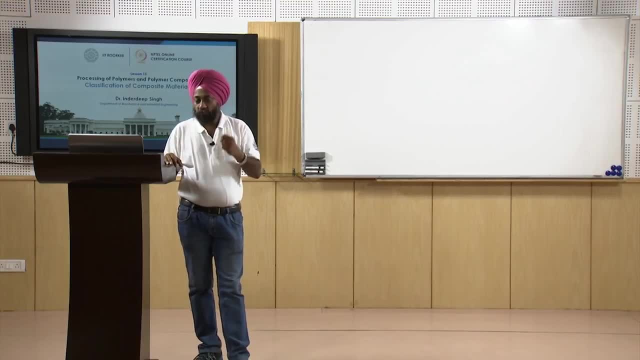 two examples should immediately come to your minds, that is, first, one is wood and second, one is the bones. so these are two naturally occurring composites, but in if you talk about the synthetic composites, it is a very big family. so, complaining about ICE composite, comes the super material, man potatoes워 might. 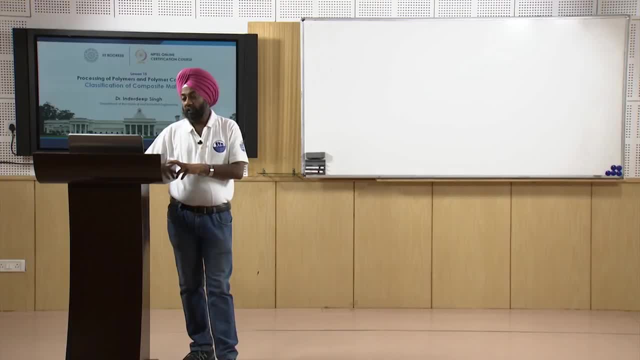 have been such a kind of non kötami RC. and still告诉 you i now this technical products, which is, as i say, over 200 different types of material, even for C THEM sometimes are beingduly wasted for bone cavings. what do you mean by non-composite polymer? these are 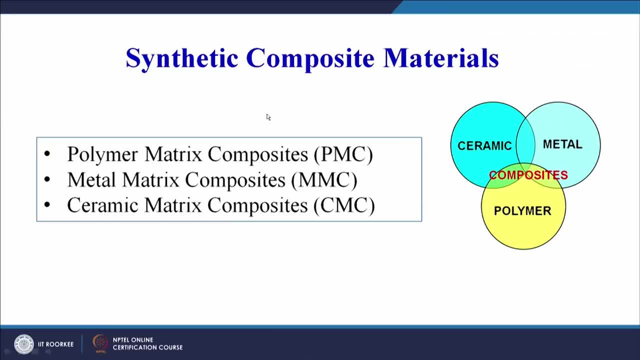 not synthetic. these are very terrible. we are making things hard. this really twice over these things this can to dig in. and then look at the iron texts that we called biological composite materials. now in this classification you can see that we can classify the composite materials based on the matrix that is used for making the composite. and here you can: 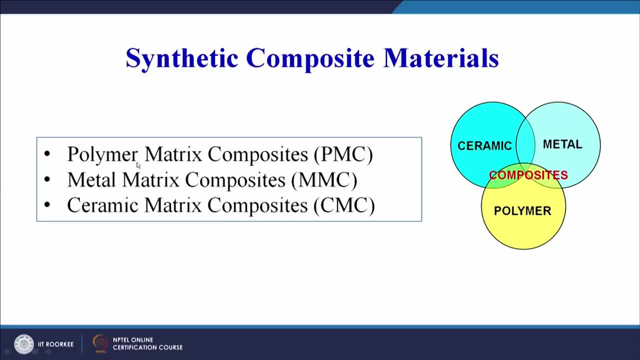 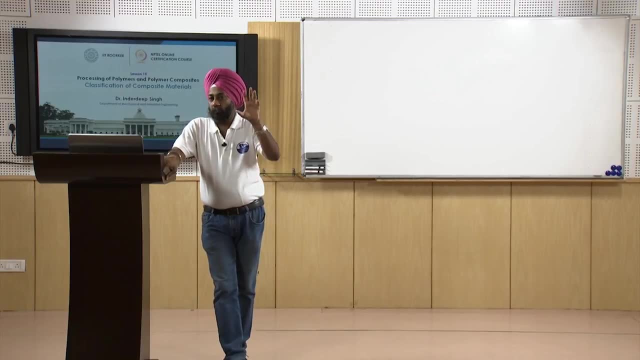 see, as the name suggests, polymer matrix composite, metal matrix composites. ceramic matrix composites. so you should remember that, based on the two constituents, you have a classification. based on the matrix, you can classify them as polymer matrix, ceramic matrix and metal matrix composites, and each one of these will have their specific application area. for example, i may ask you: 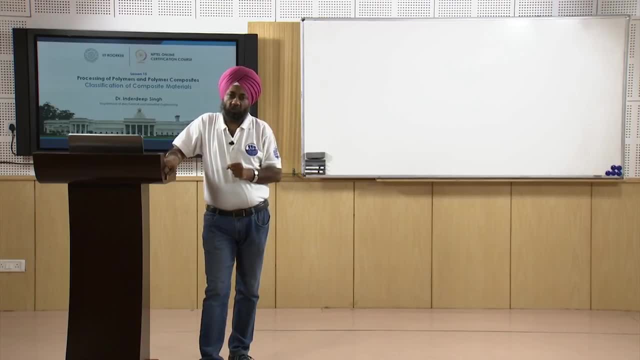 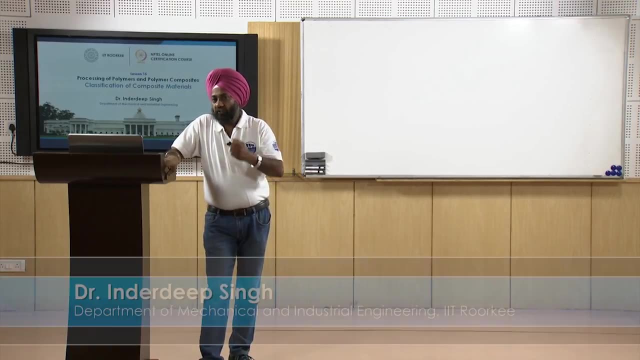 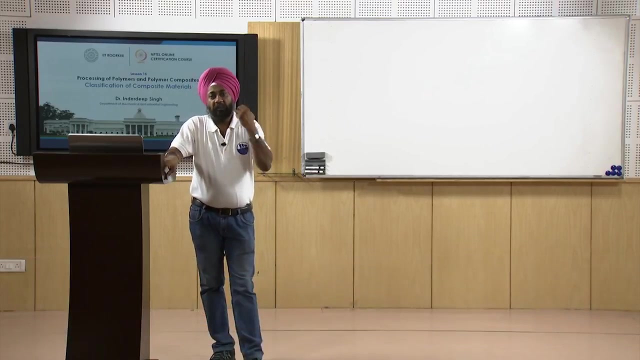 this is a common sense question, that for high temperature applications which type of composite you will suggest? now, immediately the answer should come that ceramic matrix composites. but ceramics are used for high temperature applications and if i ask you that you are using a polymer matrix composites, then you will say that for low temperature applications. 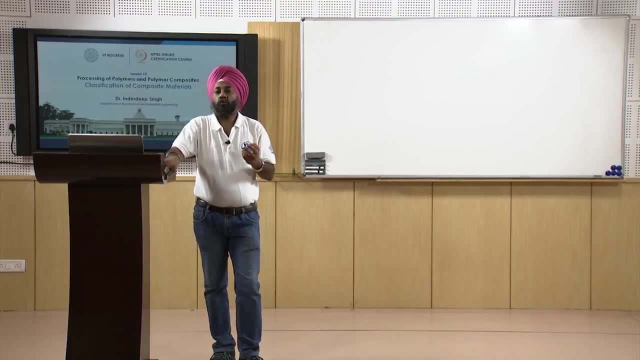 which is the composite material you will suggest immediately? the answer should be polymer matrix composite, because polymers have low melting point. they have they have very low glass transition temperature. so we have to see that what type of material is suitable for what type of application. so they, based on their application or based on the matrix that is being used, we can say: 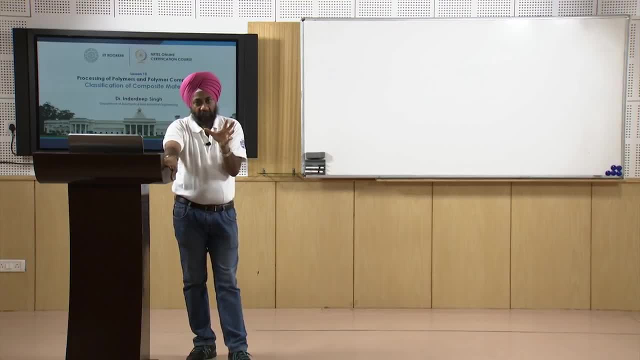 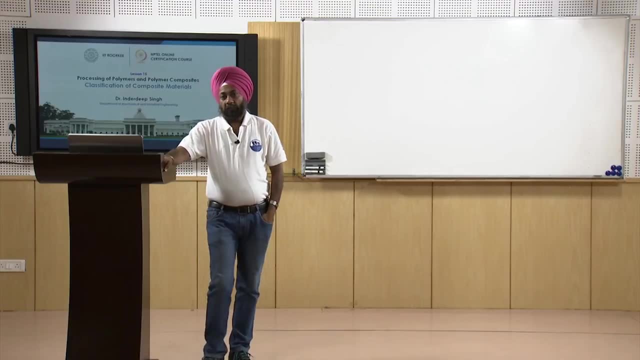 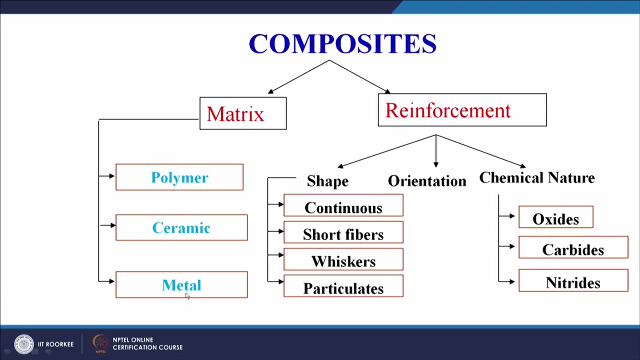 we can classify them as polymer matrix, metal matrix composites and ceramic matrix composites. based on matrix. you can see on the screen we have polymer matrix, ceramic matrix and metal matrix, but based on reinforcement. also there is a classification now based on the reinforcement. we can classify them based on. 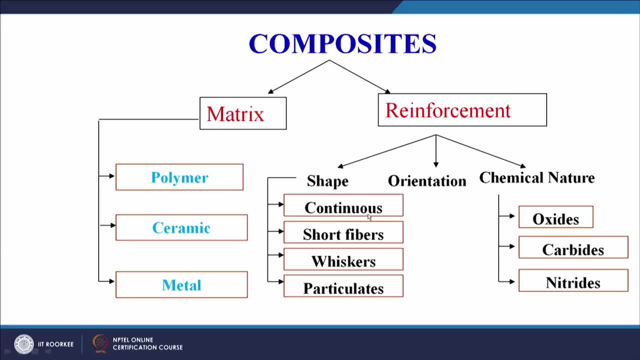 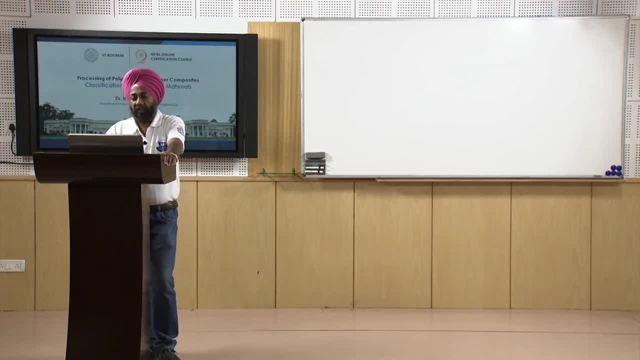 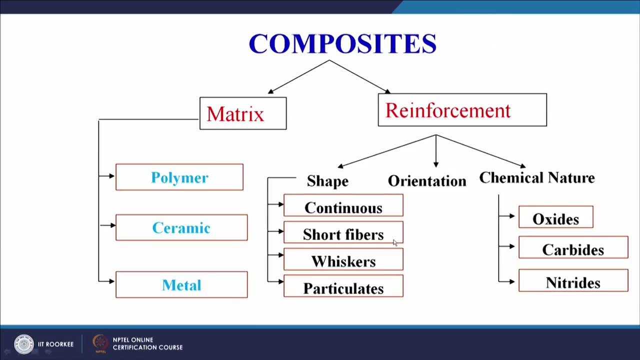 the shape of the reinforcement. now, shape can be continuous. it can be long fibers running the polymer matrix or long fibers running in a metallic matrix, so that the shape of the reinforcement can be continuous. that is one thing. then you can have short fibers in many applications, specially injection molding machine is used for making short fiber reinforced. 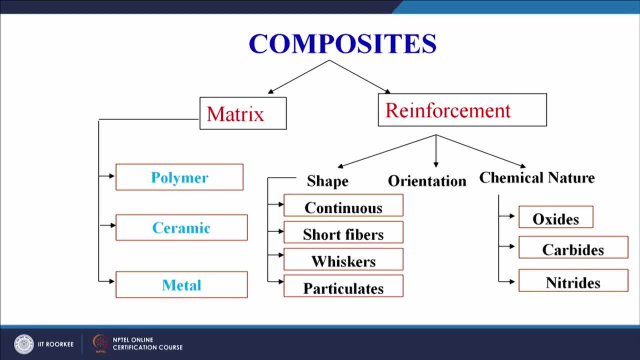 polymer composites so you can have reinforcement in the form of short fibers. you can have reinforcement in the form of whiskers. in the last class we have seen that whiskers can be randomly oriented through the matrix. whiskers can be oriented or they can be having a directional orientation within the matrix. 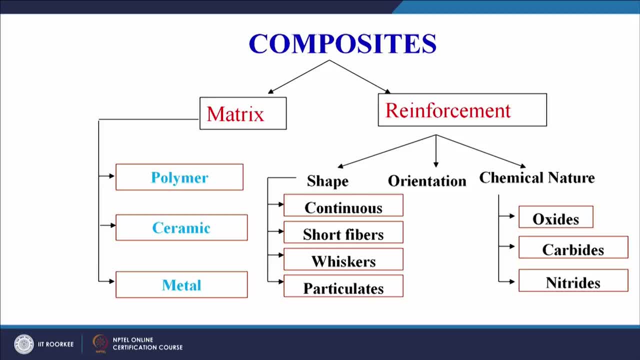 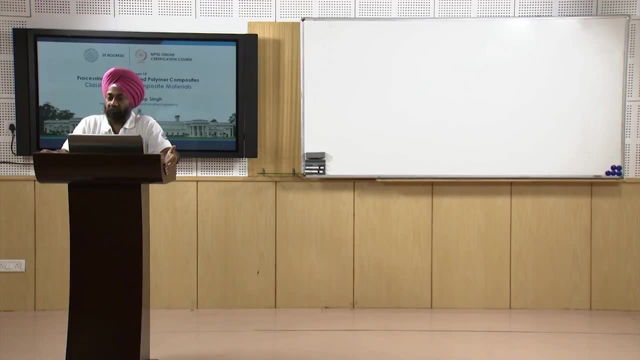 so you can have whiskers as a reinforcement. definitely they will have some aspect ratio. and finally the particulates, so you can have fine particles as the reinforcing elements or reinforcing agents in a metallic or a ceramic matrix as well as in a polymer matrix also sometimes. sometimes nanoparticles or nano reinforcements are used to reinforce the material. 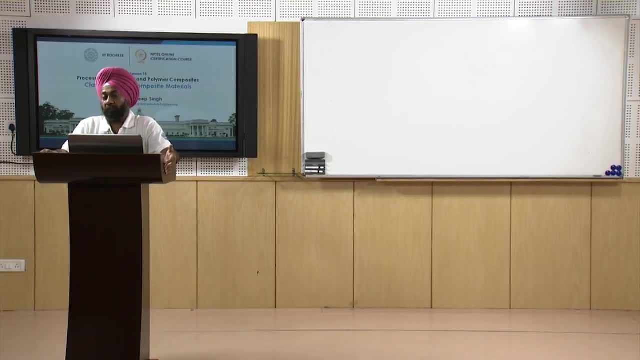 or to improve the mechanical as well as the other properties like thermal or the chemical properties. many times electrical properties can also be improved or enhanced by the addition of the reinforcement. so it is not only that reinforcement is added only for the mechanical properties or for improvement of mechanical properties. reinforcement is also sometimes added in order to improve. 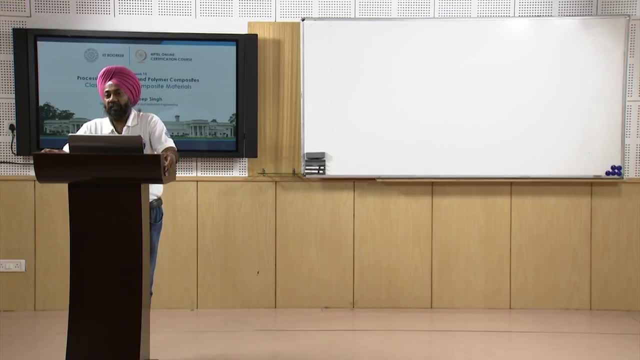 the other maybe properties such as electrical as well as thermal properties. so we can see, based on the shape of the reinforcement. we can have continuous fibres as the reinforcement, we can have short fibres, we can have whiskers, we can have particulates. so one assignment that is there for you now you should remember. 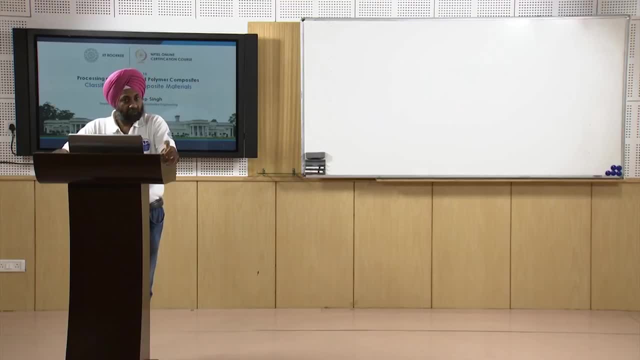 that, what is the difference between a short fibre and a whisker? that you should keep in mind and try to figure out the answer to this particular question. so what is the difference between a short fibre and a whisker? because continuous fibres absolutely clear, particles absolutely clear. so there is a grey area between the short fibres and whiskers. that 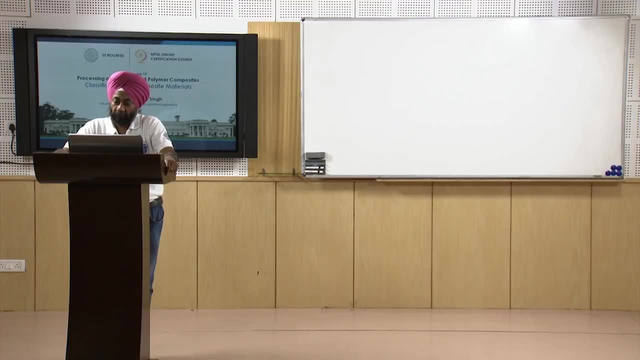 you have to figure out and find out through literature now, based on the orientation of the reinforcement in the matrix, as i have told you, you can have all fibres oriented in one direction or you can have randomly oriented fibres in the matrix. so orientation also plays a significant role in defining the properties of the resultant composite. 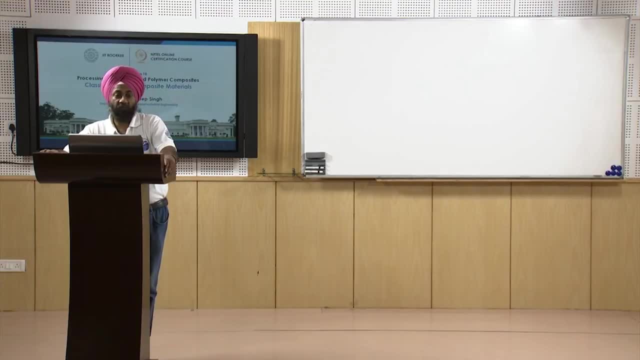 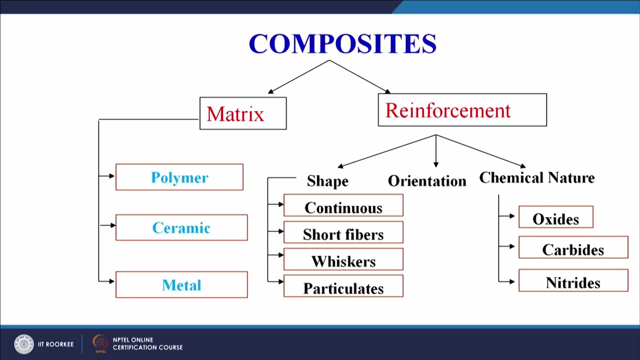 that has to be taken into account. that what is the orientation of the reinforcement? 3. Reinforcement in the matrix, similarly based on the chemical nature of the reinforcement. we can have oxide like aluminium oxide. we can have carbides like silicon carbide, as well as we can have nitrides, and this list is endless. you can have other ceramics or 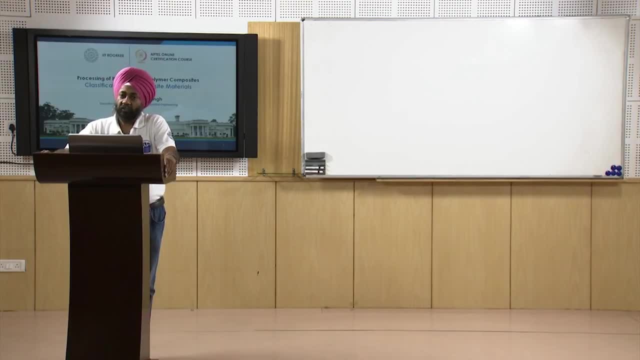 other types of materials also which can be used as the reinforcing elements. so you can see that you have a matrix which can be polymeric, which can be ceramic, which can be metallic. you have a reinforcement. 4. Composite material which can be classified based on its shape, based on its orientation. 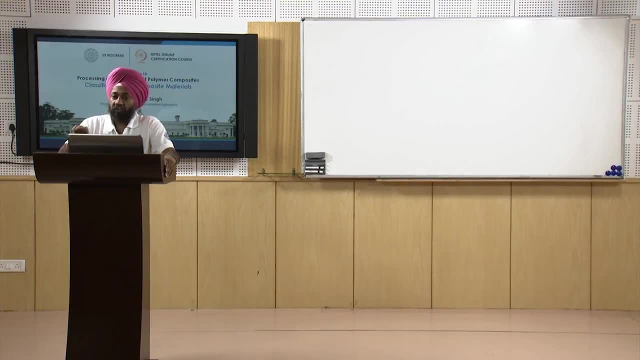 and based on its chemical nature. so this is one important classification of composite material. that is there now. simple examples can be put into this. now let us take one or two examples. the first example that comes to my mind is a glass fibre reinforced plastic- GFRP- most commonly used type of a polymer matrix composite or a fibre reinforced plastic. 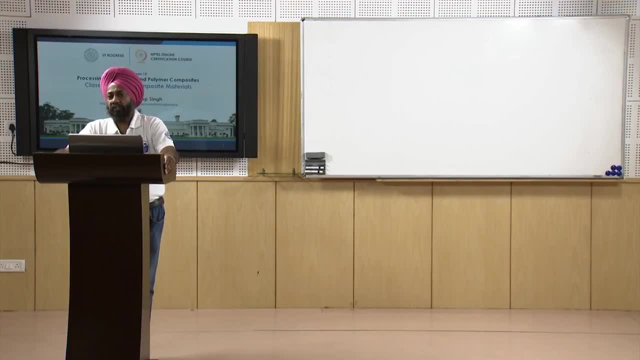 5. So these two names are used interchangeably, that is, polymer matrix composites as well as fibre reinforced plastics. now, example that we have taken is a glass fibre reinforced plastic- GFRP. now what is the matrix here? because fibres are used for reinforcing or for the 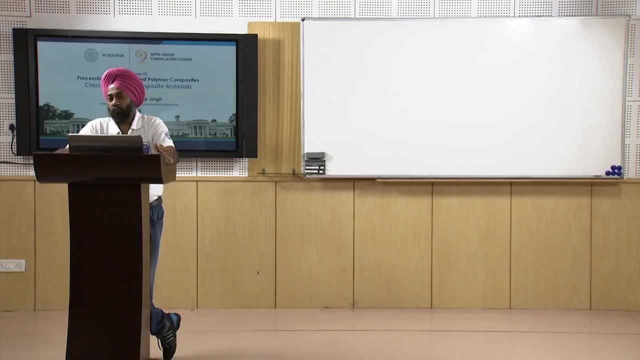 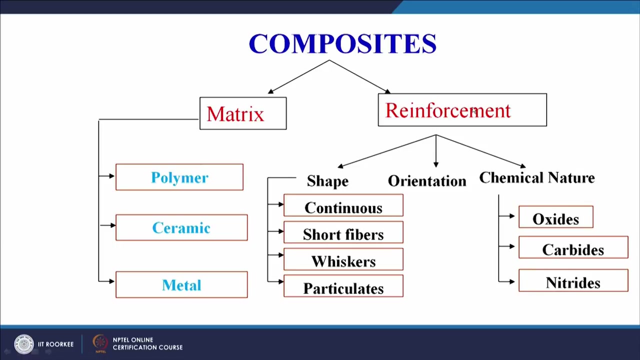 purpose of reinforcement. so glass fibre reinforced plastic means that plastic is the matrix here. so in our diagram 6. We have to see the matrix is a polymer matrix. now the reinforcement is glass fibre. the reinforcement is glass fibre. now the glass fibre can be continuous glass fibre. it can be in the form. 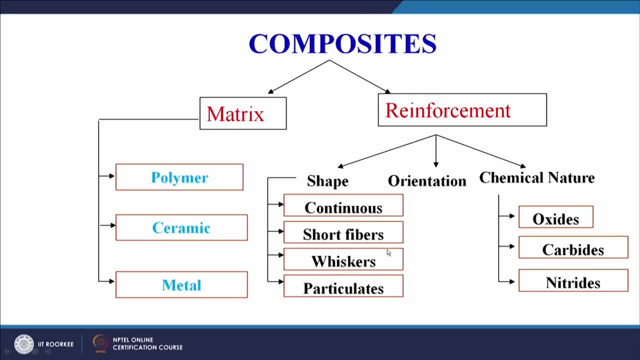 of short fibres. it can be in the form of whiskers. so we have to see that. what is the shape of the reinforcement? then the fibres are oriented. if they are long fibres, they are oriented in one direction only. we will say from the orientation point of view. 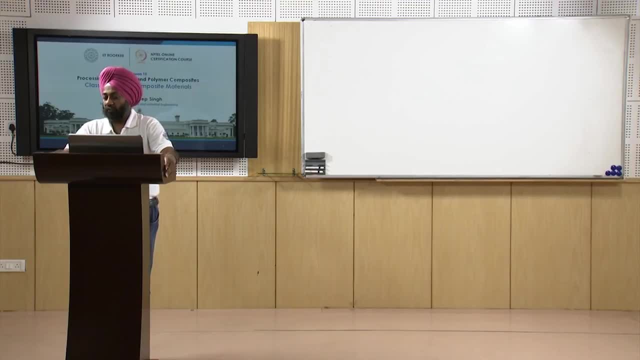 7. The reinforcement is oriented and it is in one direction only. then the chemical nature also. we can. in this case we are not bothered much about the chemical nature. but in glass fibre reinforced polymer we know that the matrix is polymer and the reinforcement is long fibres and the orientation is oriented in one particular direction. so that is one. 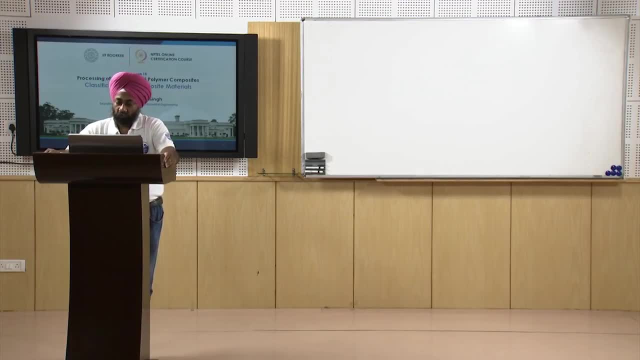 thing that has to be taken into account. so that is the broad classification 8.. Now let us take an another example of a metal matrix composite. now suppose we have aluminium as the metal, aluminium as the metal or the matrix. so your matrix is aluminium, that therefore. 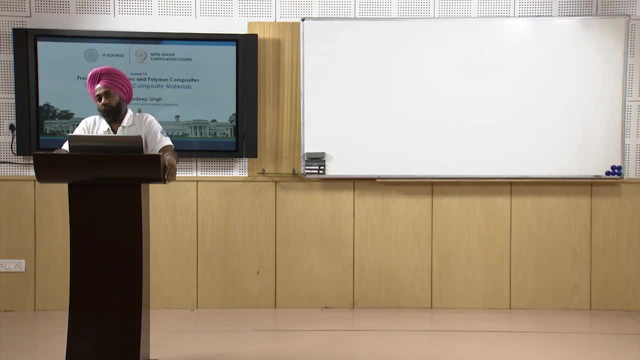 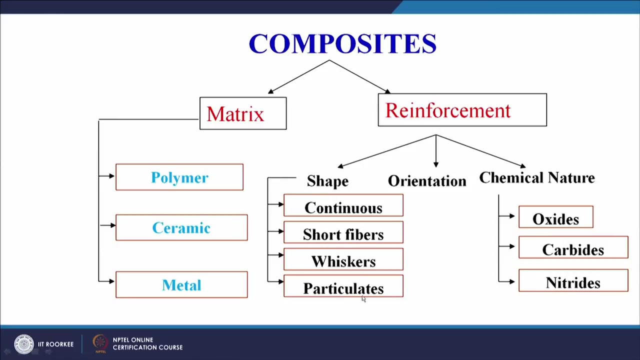 it falls under the category of metal matrix composite. now the metal is your reinforce metal is your matrix reinforcement, suppose, is silicon carbide and it is available in the particulate form. so the from the reinforcement point of view, we are taking silicon carbide. now silicon carbide. from shape point of view, we are using particles of silicon carbide. 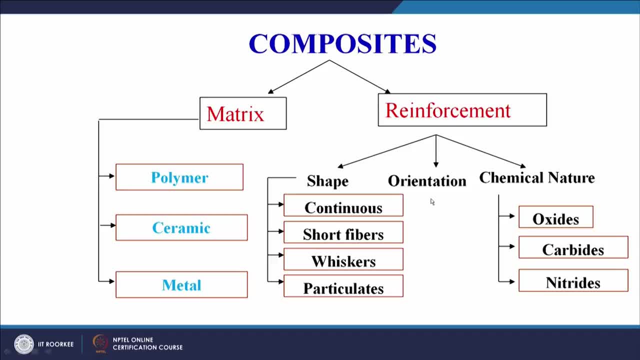 then we have orientation. we can have random orientation of the silicon carbide particles in the aluminium matrix. and finally the chemical nature. so we are using carbides, that is, silicon carbide 9.. So another example: can of metal matrix composite can be aluminium matrix composite reinforced. 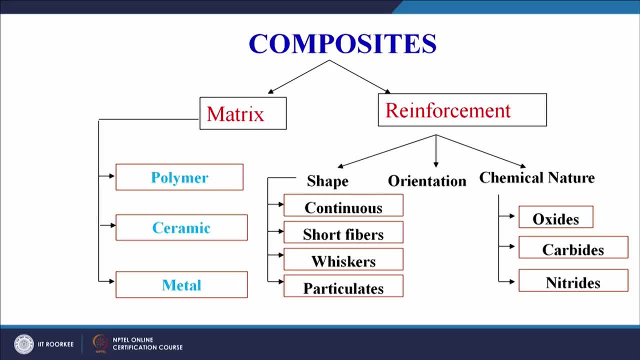 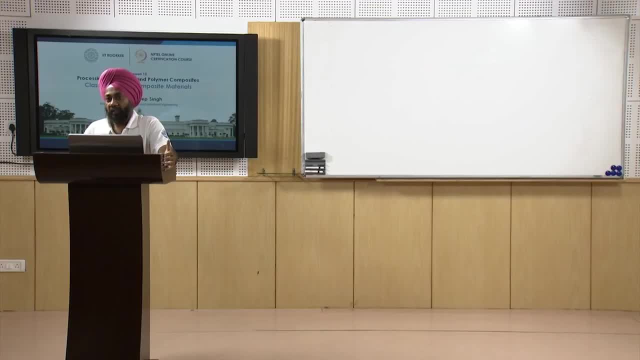 with silicon carbide or aluminium silicon carbide composite 10.. So the matrix is aluminium and the reinforcement is silicon carbide particles. so this broad classification diagram gives you so many different examples may be in the assignment you can take 5 different, you can search and you can try to figure out 5 different types of composite. 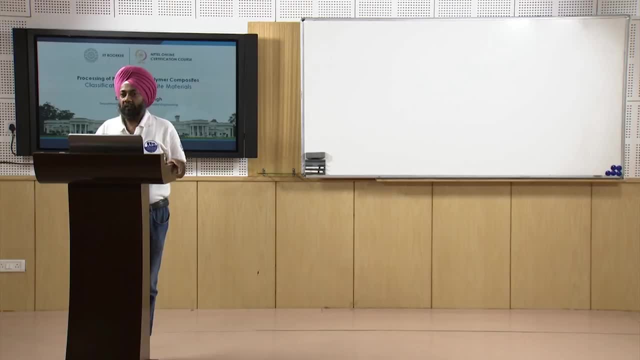 materials and then try to put them into this diagram. that what is the matrix? it is either it is polymer, or it is ceramic, or it is metal. what is the reinforcement? whether the reinforcement is based on, shape is continuous, or it is Short, or it is particle or it is whisker. then, from orientation point of view, you can: 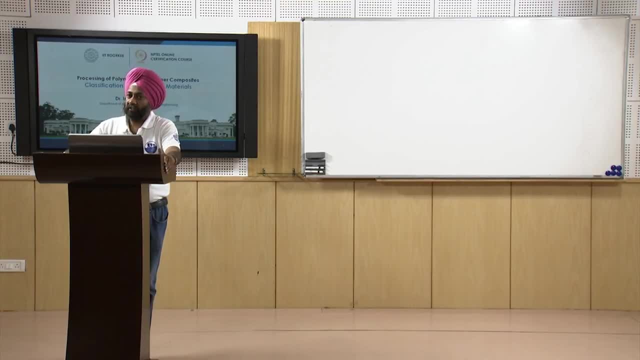 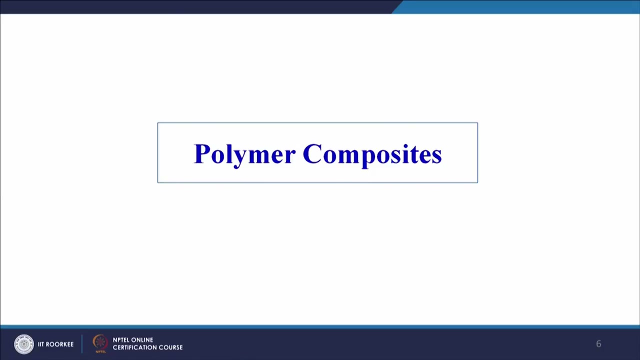 classify and then from the chemical nature point of view, you can classify. So if you do that exercise, you will be very easily able to classify the composite materials. as the title of our course is polymers, or processing of polymers and polymer composites, now we enter into the exact domain, that is, polymer composites. 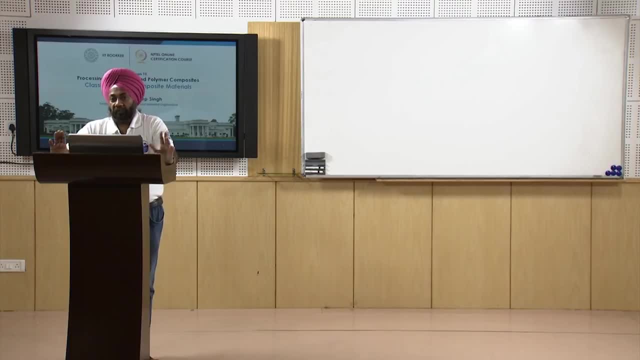 11.. As I have told you, these composites, basically polymer based composites, are also called fibre reinforced plastics, because the matrix is plastic or polymer and reinforcement is in the form of fibres, specially in case of polymer based composites. So we usually call them fibre reinforced polymer composites. also- and here again we can see the 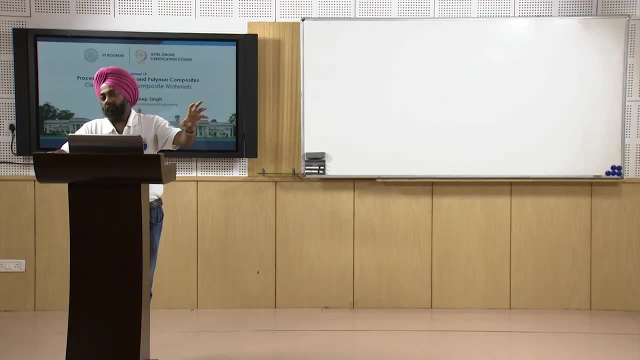 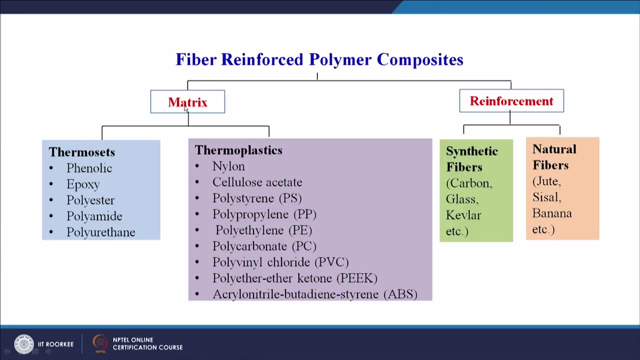 examples, as I have told you are. the last diagram was a generic diagram, a general diagram, classification showing classification of composite material 12.. But this is a specific diagram related to the polymer based composites. only so we can see from matrix point of view. we can have two types of polymers. one are thermosets and 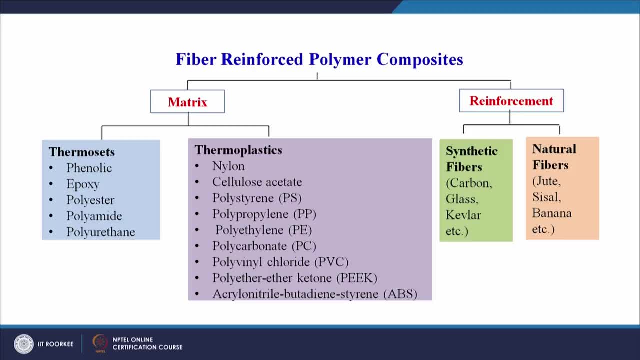 the thermoplastic, and this we have already covered in our course in the very beginning my, I think in the second or the third session. So thermosets can be epoxy, polyester, polyamide. thermoplastics can be polypropylene, polyethylene, polyvinyl chloride, polyether, ether, ketone or ABS, that is, acronitrile butadiene. 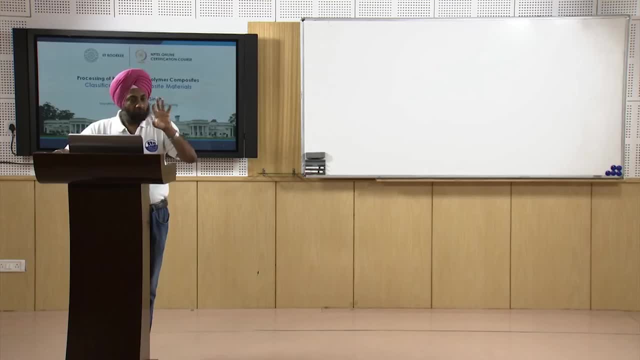 So we can have a thermoset matrix or a thermoplastic matrix, and must I address this point that, depending upon the type of matrix, our properties will be different. you have a thermosetting matrix, the properties will be different. you have a thermoplastic matrix, the properties 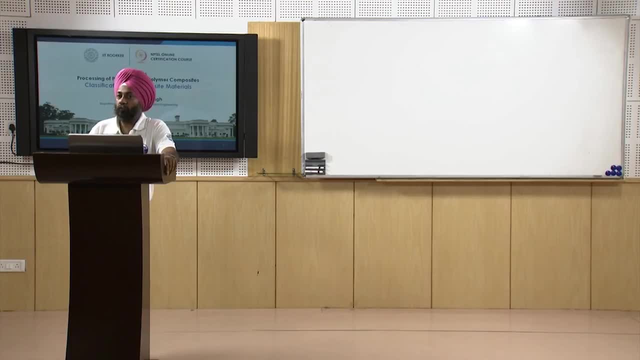 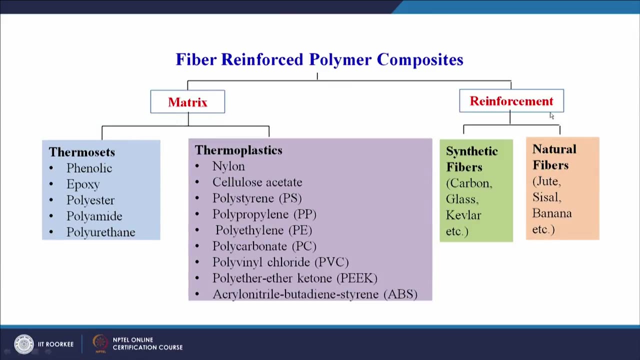 will be different. so, from matrix point of view, in case of polymer composites, we can have thermosets and thermoplastic. similarly, from reinforcement point of view, we can use synthetic fibres, So we can have carbon, glass, Kevlar as the reinforcement, and we can also use the natural. 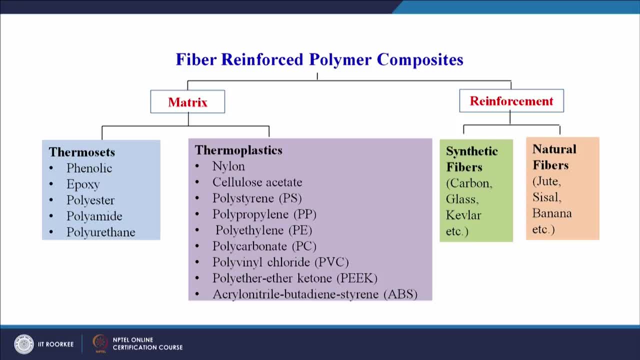 fibres as the reinforcement. from synthetic fibres point of view we can have carbon glass, Kevlar as the reinforcement, So Kevlar is basically aramid fibre. so the synthetic fibres, carbon glass and Kevlar. from the natural fibre side we can have natural fibre is a long list and we will try to address. 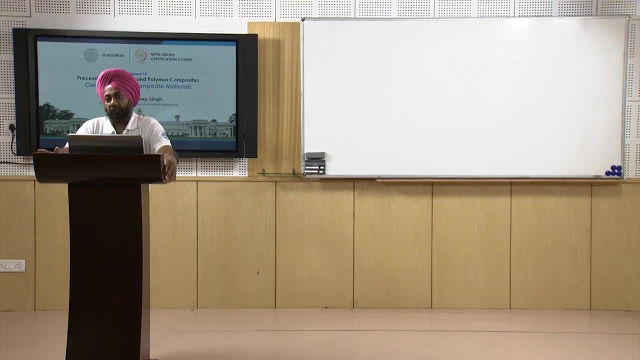 it, if possible, in our course. what are the type of different types of natural fibres, how they can be classified, how they are derived, what are the sources of different types of naturally occurring fibres? But okay, from just to introduce the concept of polymer composites we can have matrix that 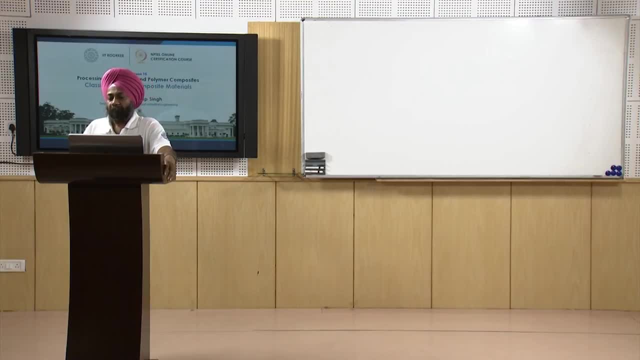 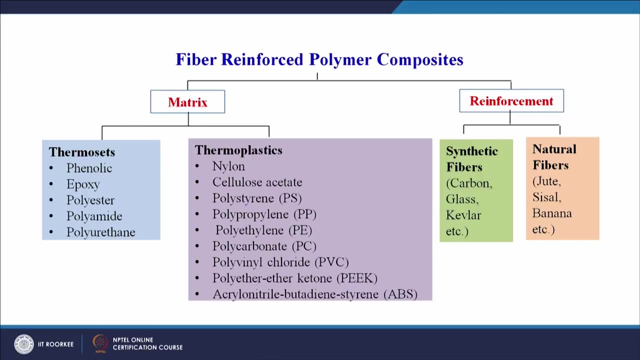 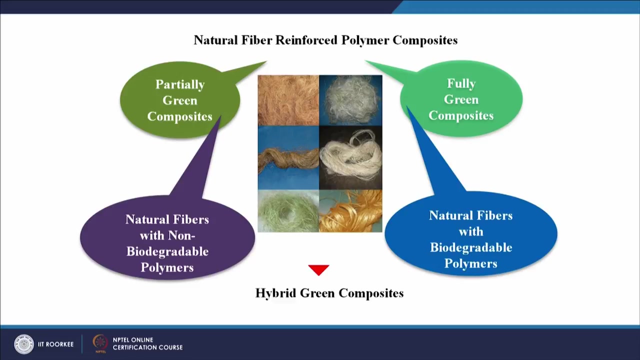 is thermosets or thermoplastic, and we can have reinforcement, that is a synthetic fibre and a natural fibre. from natural fibre. mostly occurring are jute, banana, sisal fibre. Then again we have- we can have natural fibre reinforced polymer composites also, in which the natural fibres are used as reinforcement. 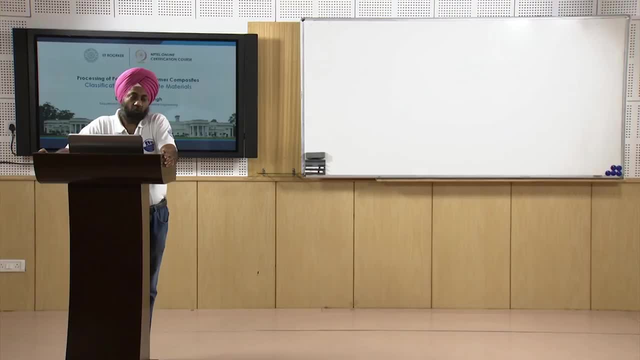 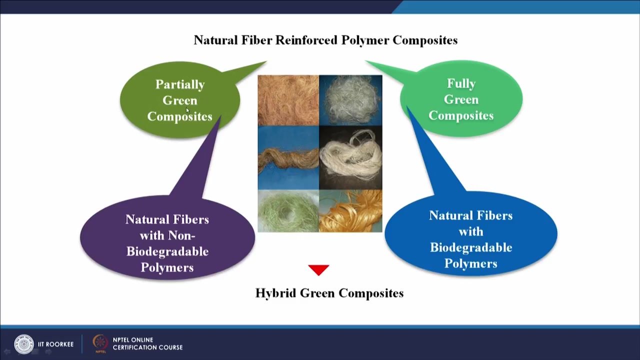 and we all around the world. there is a trend towards biodegradable composites in which the polymer or the matrix is also biodegradable as well as the fibres or the reinforcing members are also biodegradable. So natural fibre, reinforced polymer composites we can see here we can have partially green. 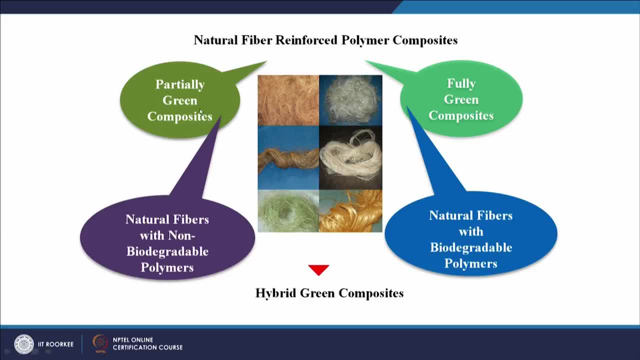 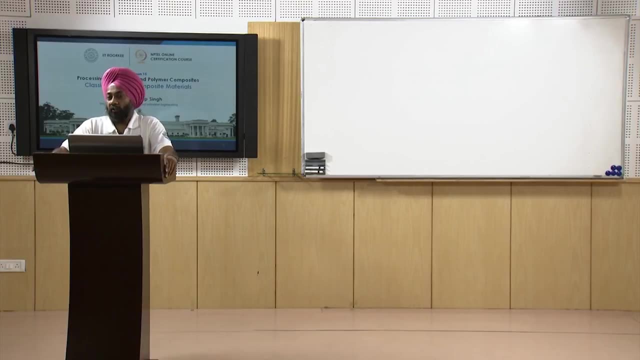 composites we can have. in partially green composites we will have natural fibres with non-biodegradable polymers. So the reinforcing agent, that is, the fibres, are biodegradable or naturally occurring, but the polymer or the matrix is not biodegradable. it is a synthetic matrix, as we have seen in. 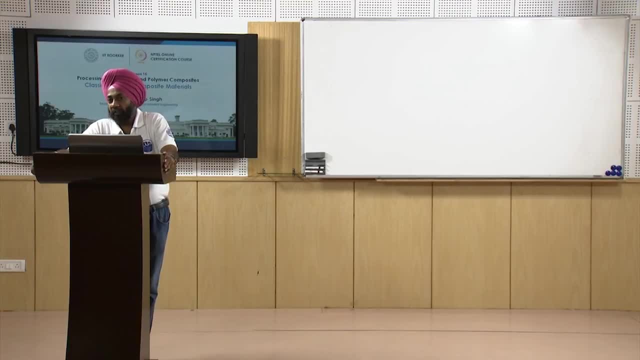 our previous slide that thermoset and thermoplastic matrices are there. Suppose we use a thermoset and we use epoxy as the matrix, so it is non-biodegradable. If we use thermoplastic and we use polypropylene or polyethylene as a matrix material, it will. 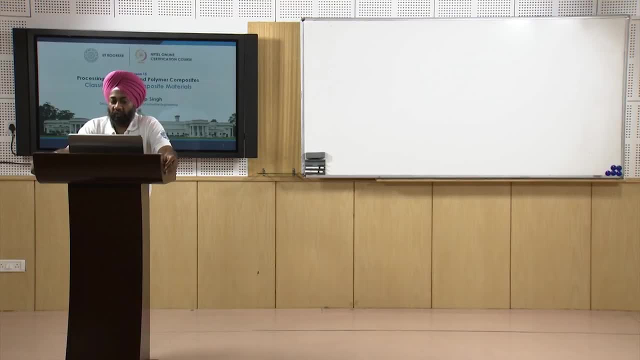 it is non-biodegradable, but the fibres actually are biodegradable. So then we get partially green composites. but what is the trend? The trend is towards fully green composites. So for fully green composites, we should have natural fibres with biodegradable polymers. 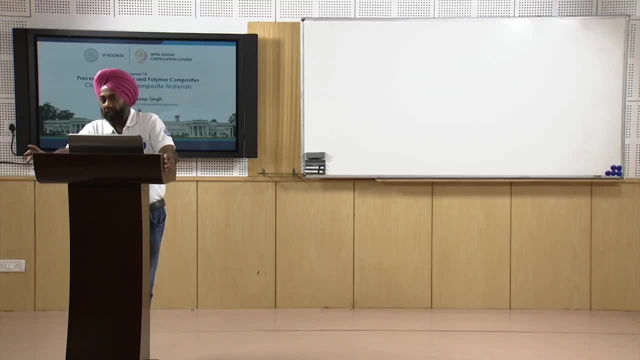 So our polymer or the matrix should also be biodegradable, our fibres should also be naturally occurring and then we can have hybrid green composites. that is another category of composites. So broadly we can say, if we use natural fibre as the reinforcement we can at least get partially. biodegradable composites, and if we can have the liberty of choosing the matrix material also, which is biodegradable or a biopolymer, then we can have the advantage of making a fully biodegradable composite material, because the reinforcement material is also naturally occurring or derived from nature. 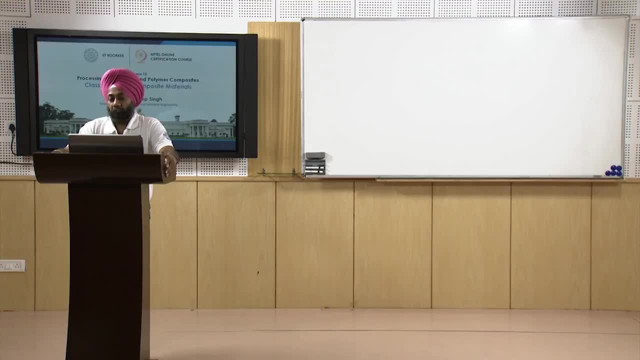 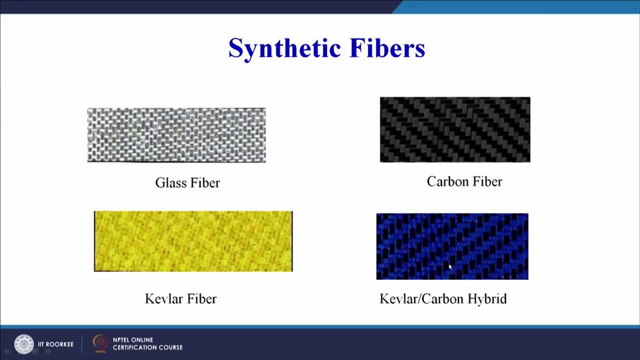 Now on your screen you can see the different types of synthetic fibres. you can have glass fibre, the Kevlar fibre, Kevlar carbon hybrid fibre, in which in one direction we have maybe black portion is the carbon fibre, the blue portion is the Kevlar fibre. 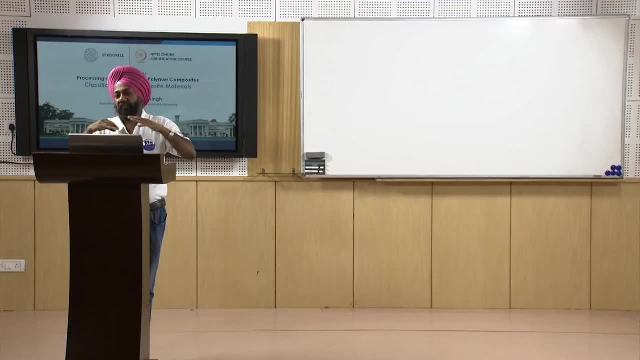 So we can have hybrid also in the one in one direction and the other direction, longitudinal, and the transverse. basically this is called warp and weft in textile technology, that in one direction The fibre is called warp and another direction of the fibres is called weft. 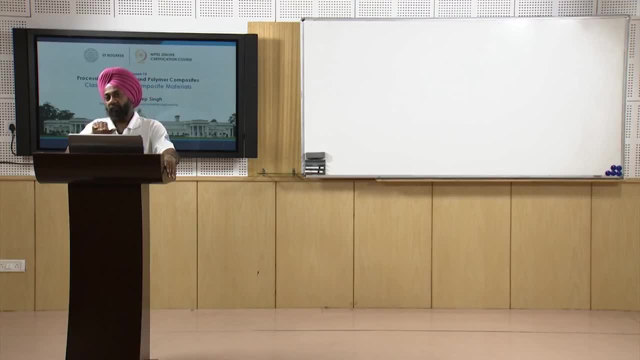 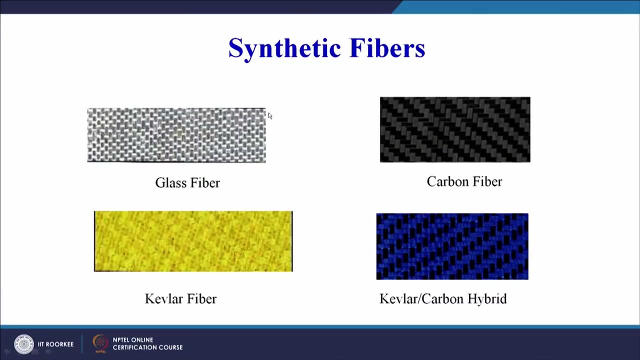 So here we can have different fibres in warp and different fibres in weft, So that basically gives us a hybrid type of fibres which can be used as a reinforcement in case of polymer composites, and we can have neat carbon fibres- woven carbon fibres- woven. 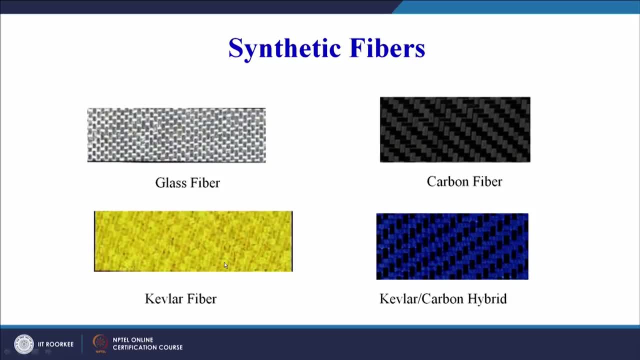 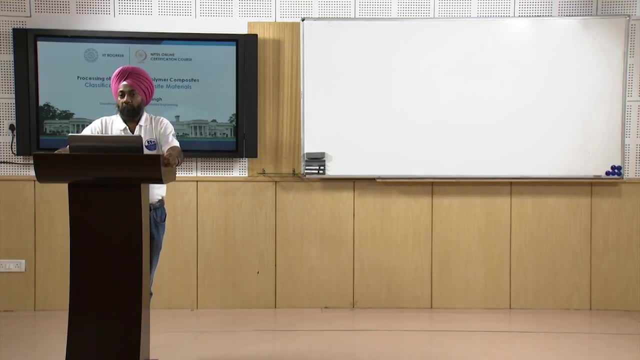 glass fibres, woven Kevlar fibres. so this is all. these are synthetic fibres and these days, even people- People- are trying to attract or to get the best properties. people are taking natural fibre in one direction- maybe warp or weft- and the synthetic fibre in other direction. 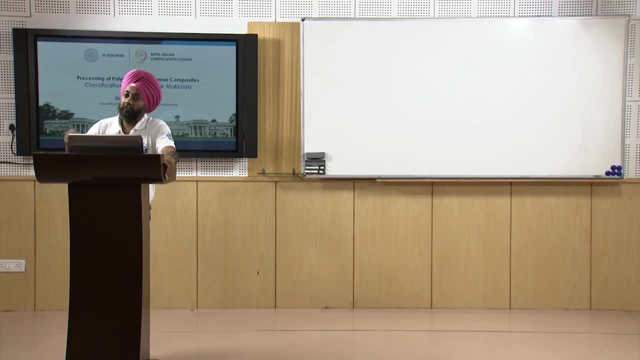 that is also possible and that type of hybrid layer, hybrid fibres, are also available which can be used as reinforcement, for reinforcing the polymer matrix. so lot of research work is going on, even the weaving pattern. people are working all around the globe to find out that. 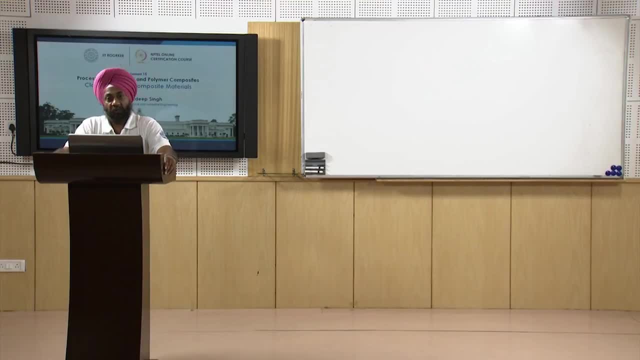 What is the best weaving pattern for a particular combination of fibre so that we get the best properties when we use these as the reinforcing elements or reinforcing members in polymer based composites? On your screen, this is a list showing different types of natural fibres. they are there in: 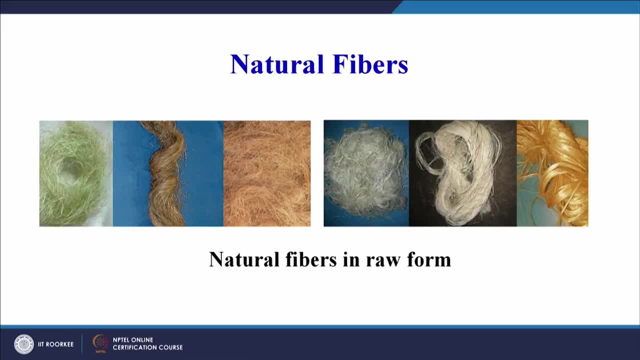 the raw form. they can be woven into the matte form and then the matte can be used as a reinforcement for making natural fibre reinforced laminated composites. but this is just showing the raw type of fibres. These are the natural fibres which are available and these are. these have been derived from. 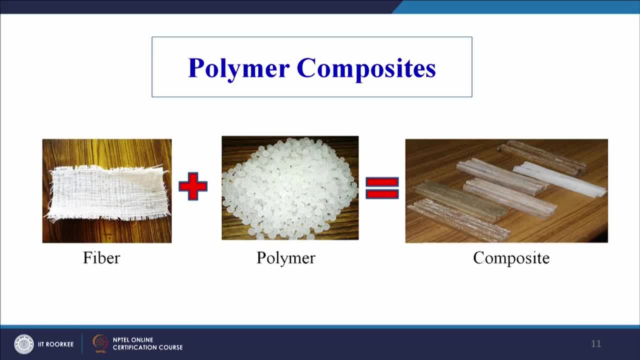 nature And once we have the natural fibres, we have the polymers which are readily available, we can make a composite material. on your screen you can see the fibre, when the raw fibre which was shown in the previous form, when it is woven in the form of a matte, this is a woven. 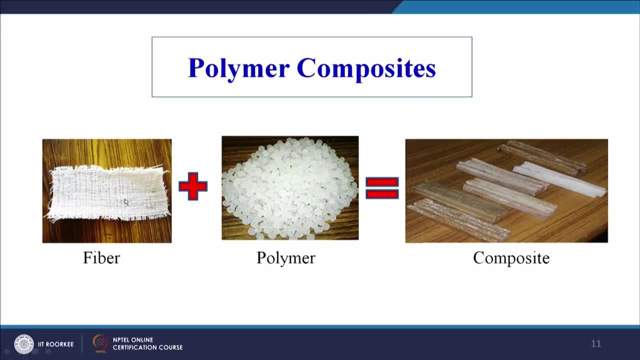 natural fibre matte and this can be used as a reinforcement agent, and this is a polymer pellets, thermoplastic polymer pellets. When we combine them together, we can make engineering materials like this, and these are the composite materials which can be used for various engineering applications. 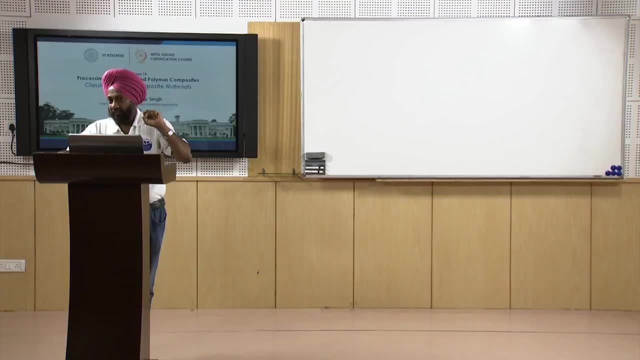 So here we can see, the natural fibre is acting as a reinforcement member for the polymer and we are making a composite material, and the composite on your screen is shown here. So you can see that a fibre and a polymer have combined together to make a third material. 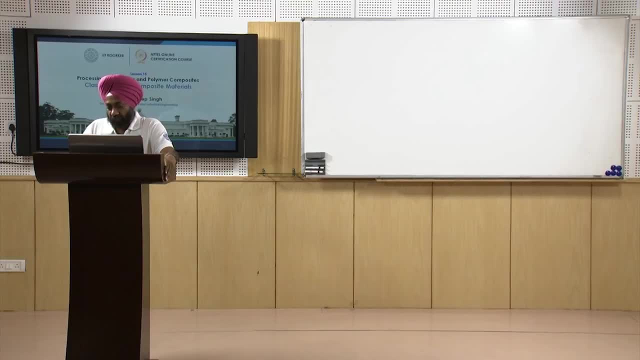 which can be used for various engineering applications. So this is, I think, the end of today's session. So we have tried to classify the composite materials based on the matrix. we have tried to classify the material based on the reinforcement. we have taken some examples that in this classification. 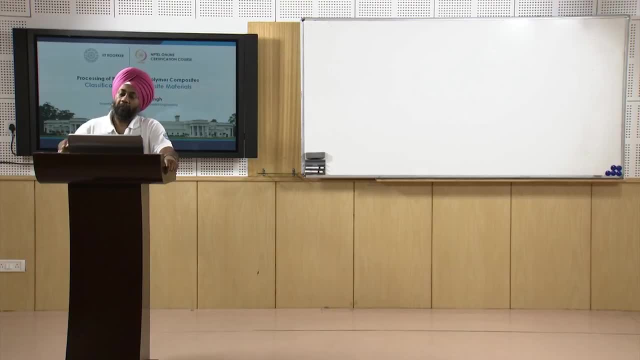 where which example can be we can fit in. and then we have tried to understand what are the different types of synthetic fibres. we have seen what are the different types of natural fibres And how they can be used for combining them with the polymers to make them a composite. 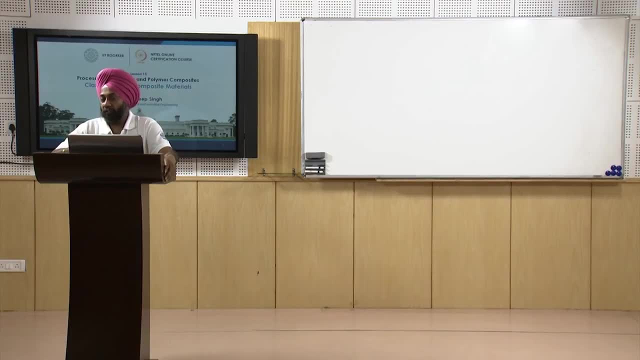 material. I think now the classification is absolutely clear to you and we have taken a slight step towards our topic, that is, processing of polymer composites. by classifying the polymer based composite, we have seen what is the matrix: it can be thermoset, it can be thermoplastic. 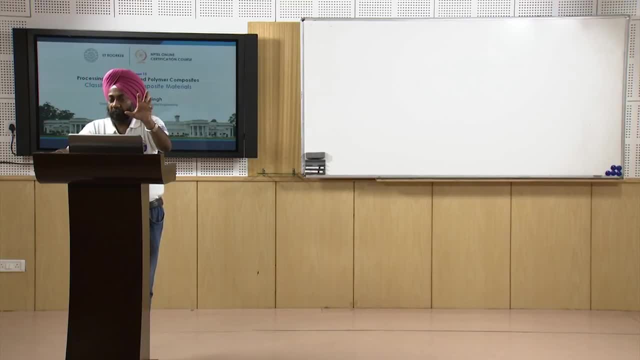 we have seen what can be the reinforcement. we have seen synthetic fibres as reinforcement. we have seen natural fibres as reinforcement. now we will see. the last slide gives us a glimpse as well as sets ah background for our further discussion, because now we have to understand that this plus sign, which is 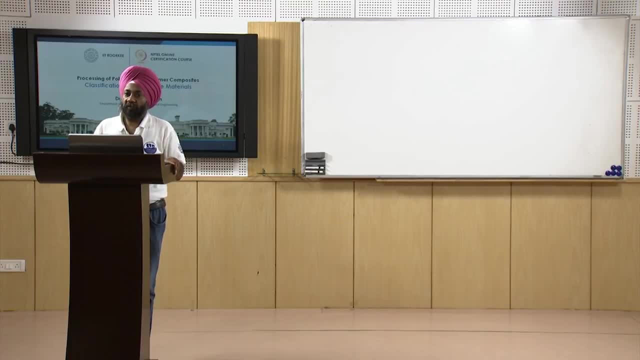 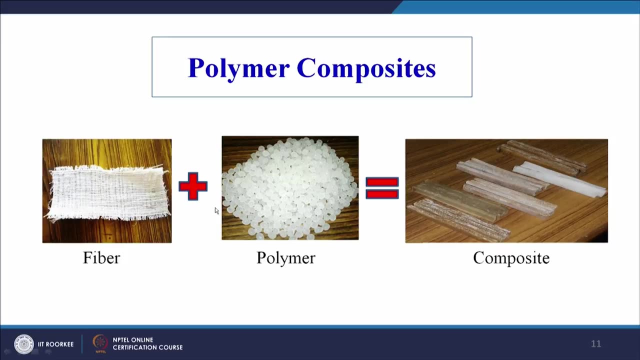 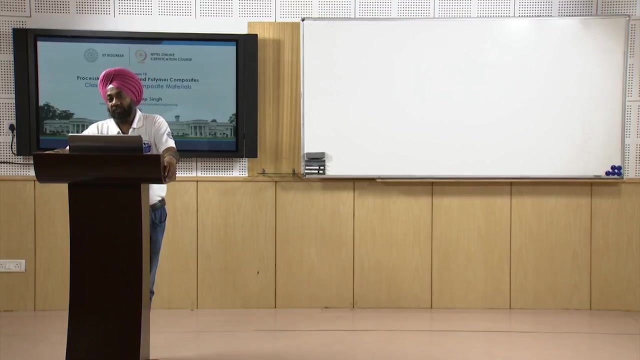 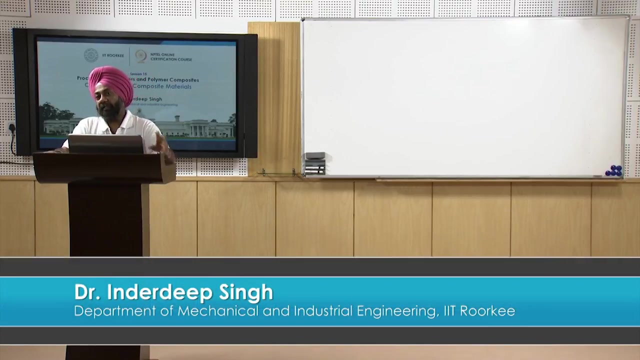 on your screen. this plus sign seems to be very, very simple, but the colour signifies its importance: that how now we can combine this fibre and the polymer together to make this composite material. so the whole discussion here on will focus on the processing roots, technologies, techniques for combining the fibre and the polymer into a composite. so 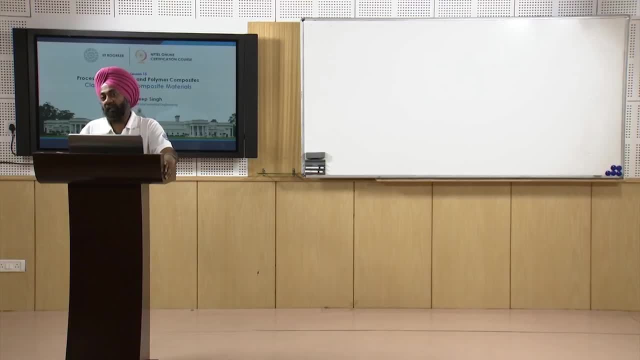 that the properties that we get, that we have planned that we have, that we have designed the properties that we are able to get by adopting the best possible technique for combining the fibre and the polymer together, and the classification or the processing will depend on a number of parameters which will will. 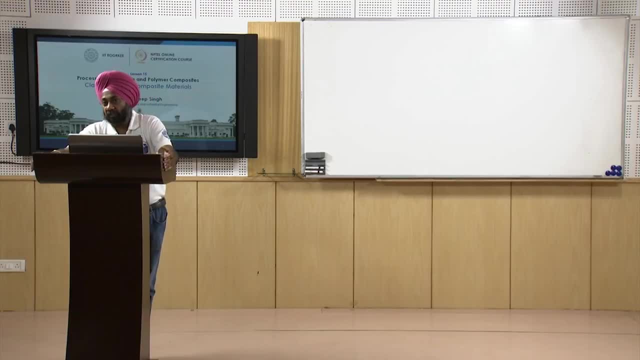 be, which we will be discussing one by one, stage by stage, phase by phase, in our subsequent sessions. so with this we come to the end of today's session on classification of composite materials. thank you.